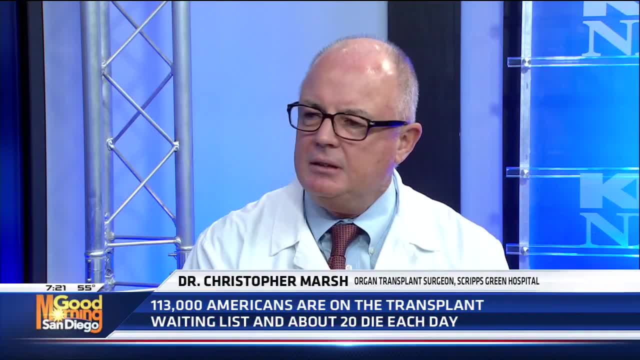 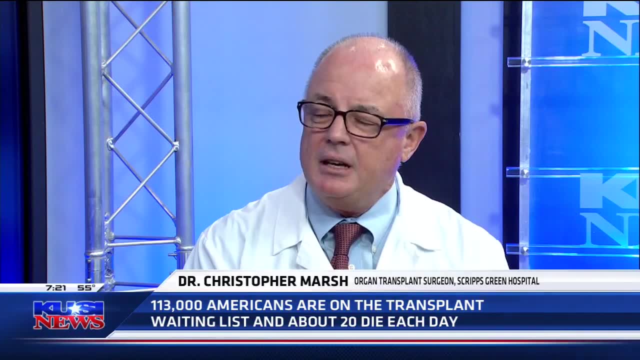 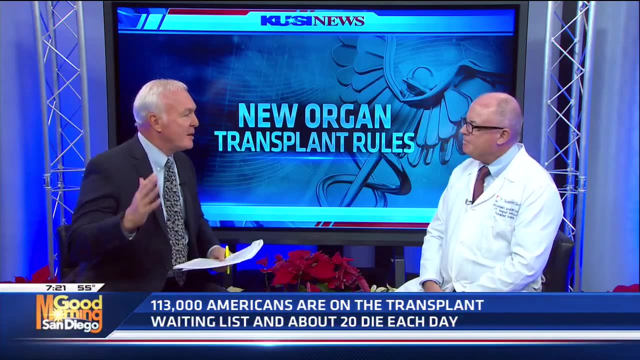 organs that are just not being recovered, and we need organs to be recovered. there's about a hundred and thirteen thousand people on the list and, as it stands now, about 20 die a day without an organ, so the demand for organs exceeds the demand of people who are passing away or involved. 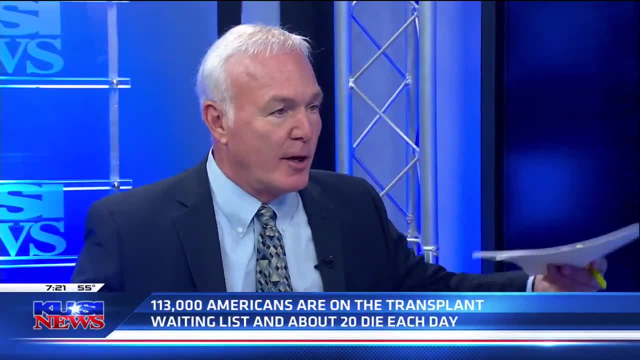 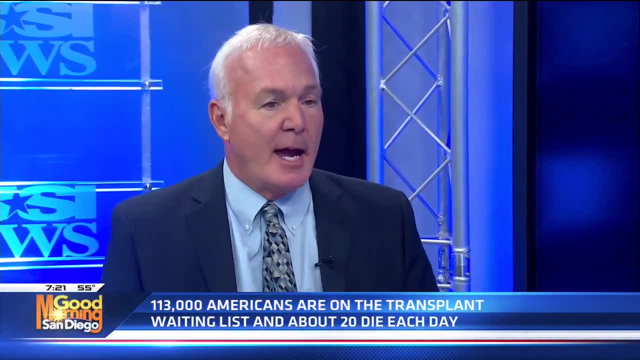 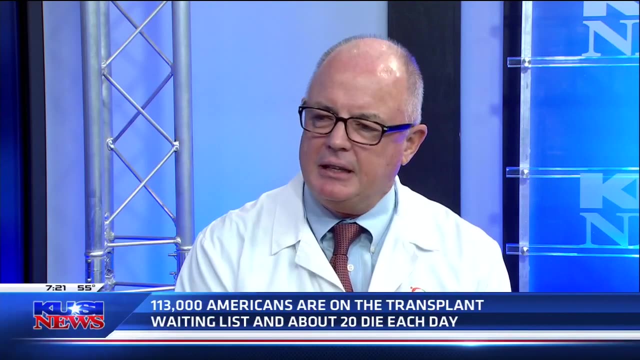 in accidents that can provide organs. the two categories are out of sync. right there they're out of sync. so you need to have living donors participate. we do now. unfortunately there's- you know, there's 7,000 live donors being done out of the 36,000 a. 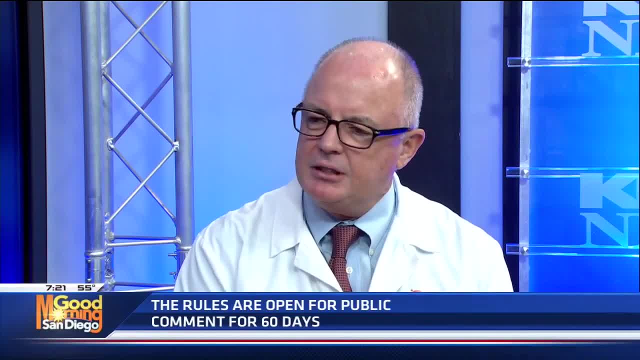 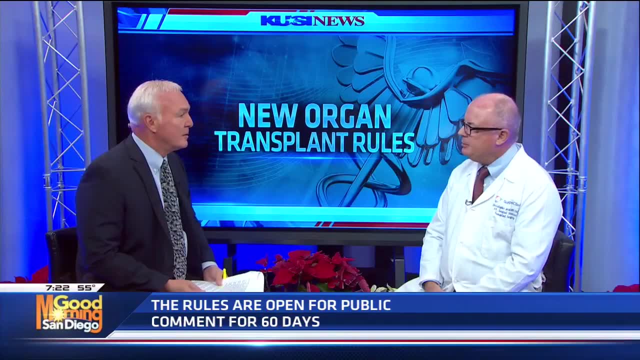 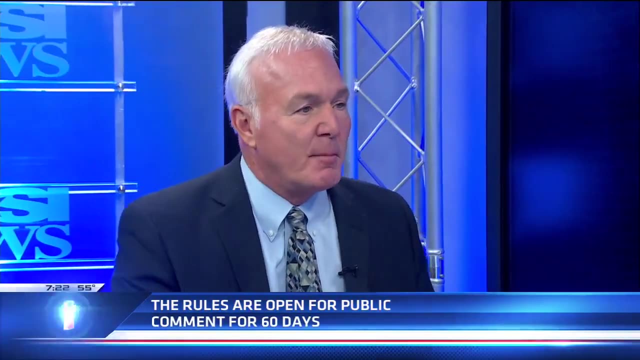 year, but any incremental increase is going to is needed and this, these we think, will help. these changes are impactful, then correct, yes, they should be. anything to save a life is intact, all right. what talk about from a medical perspective people? obviously, if it's somebody in your family or that you match up well with, I don't think anyone. 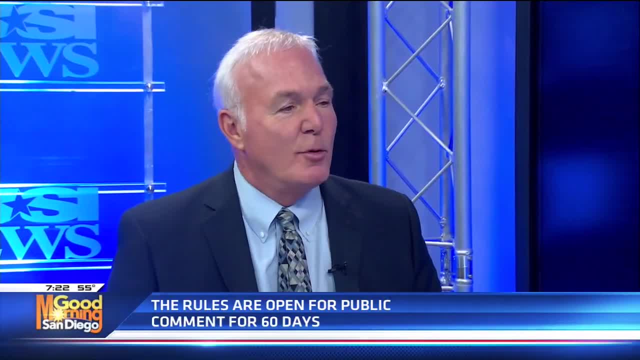 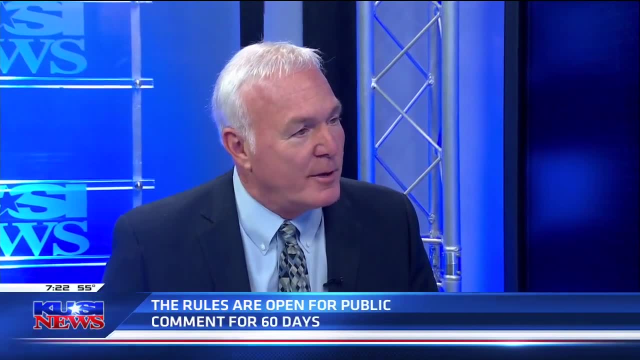 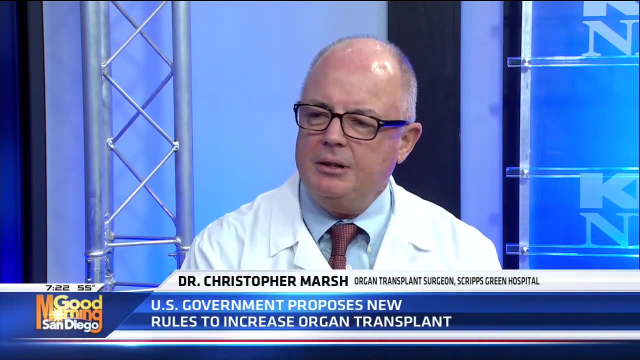 raises an eye to but say: people who are down on their luck financially and now are going to be selling their organs as can you as a doctor, are you okay with that? well, I don't think we're going there yet, I mean, but I think there does need to be an increased awareness about the, the opportunity. 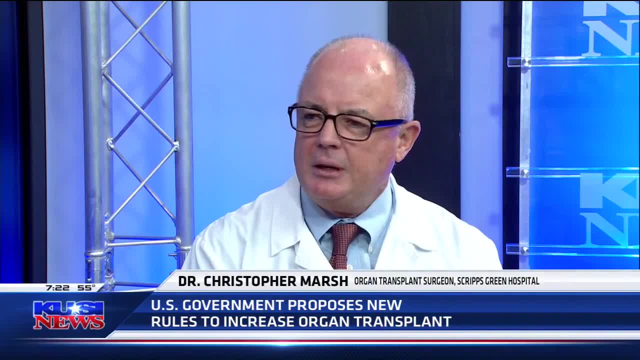 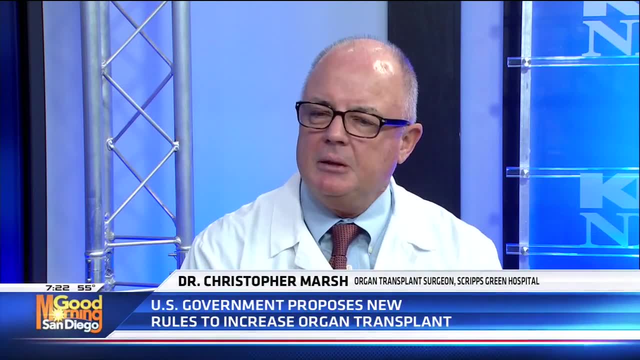 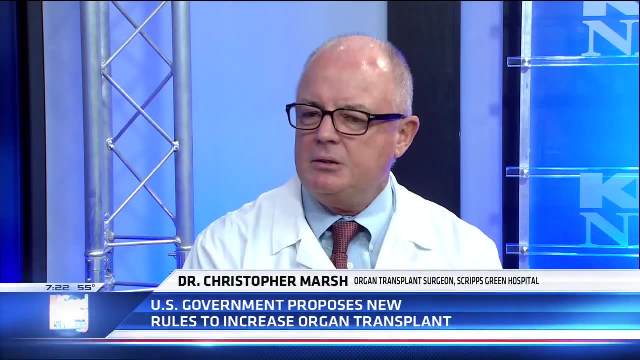 and we've had individuals who just want to do the right thing and be an altruistic donor. but again, we're trying to take this incentives away. so people will be willing to do it and there's many reasons, but increasing awareness of living donation will help. we think these regulations will help. it will. 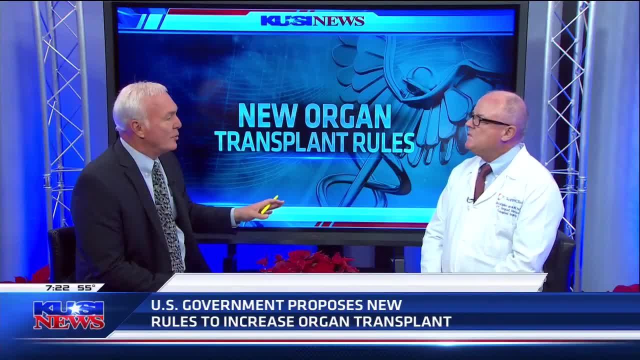 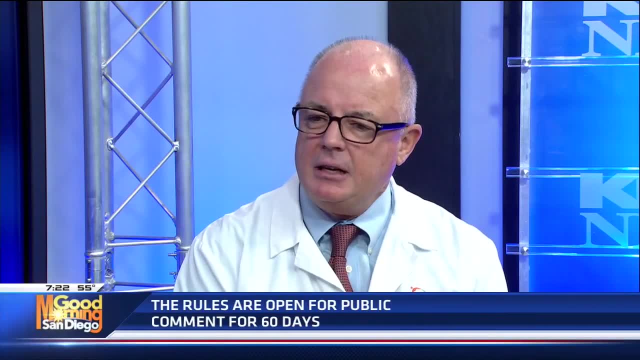 know see how it plays out. so give us a timeline of these new rules. are they in effect immediately or no? no, they're about. are they sick? being proposed? they're, they're there and there's a six day, 60 day period where they're out there for comment and then they go into effect. so it'll occur. 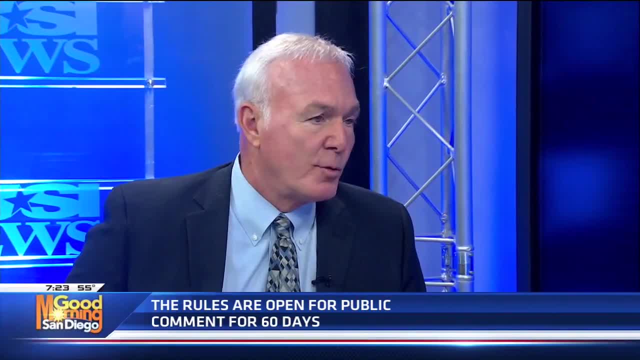 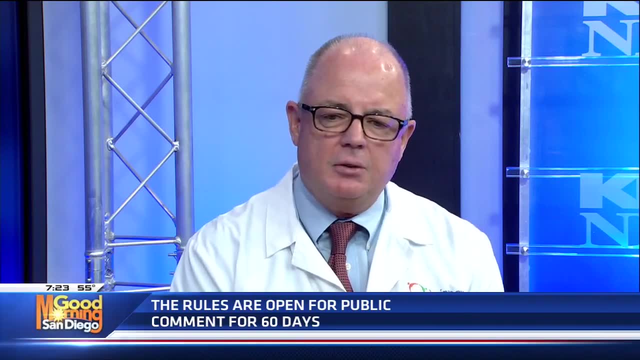 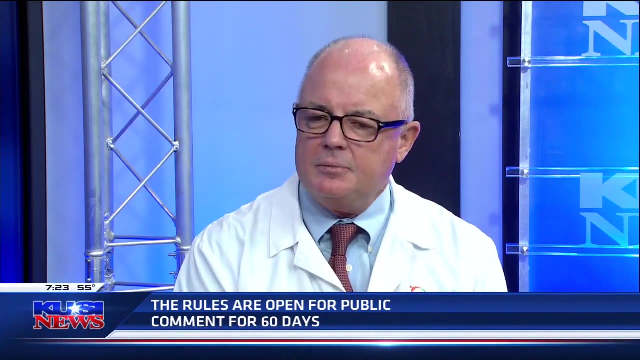 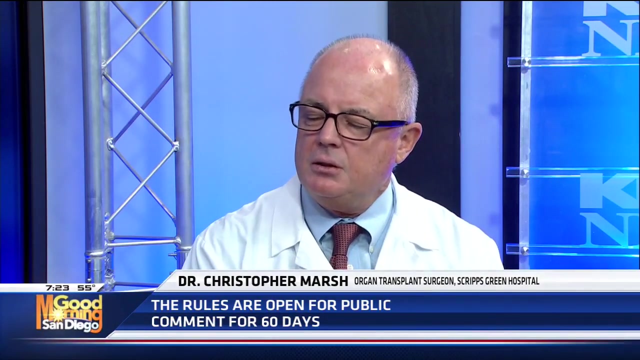 soon actually. so what else besides these laws and rules changes? what else is out there that can you admit that from the effort we tried to generate in the sense ofQU FIRST, LET'S Schridoq, THE FaC satellite, and that the to so the cause for a depression is central to a home health communication? one of those at the 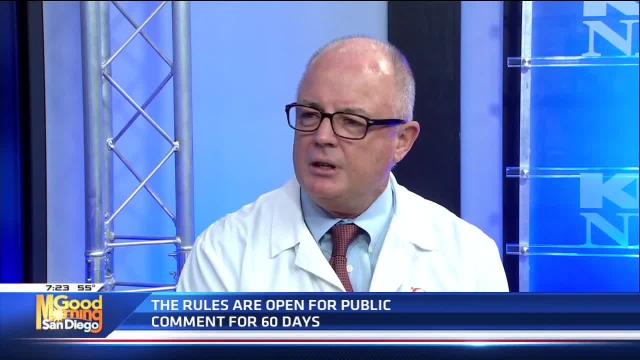 stock room important because, for the main reasons, why would we leave home? because what are we doing to use more? that's a good question. so right now, other than living donors, we are looking at a variety. The cure rate with the new drugs is phenomenal. So if you can get an organ and not die, 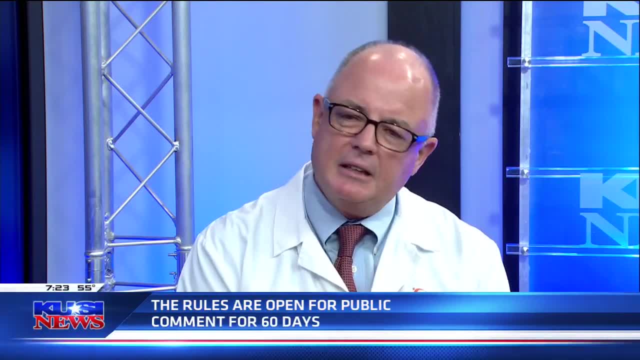 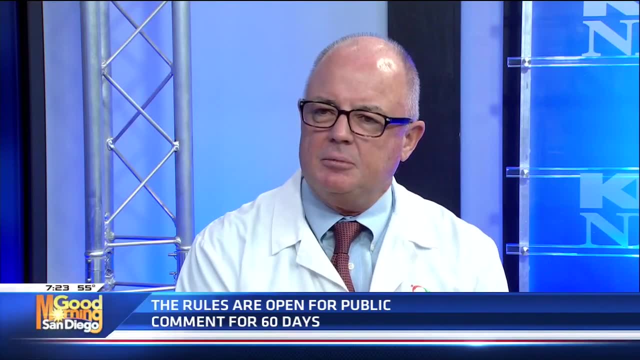 you've just saved your life by taking that type of organ. And the last is older donors. So we're using more older donors and putting them in. older patients: Transplant programs have been historically conservative for their outcomes. but if you're too conservative, 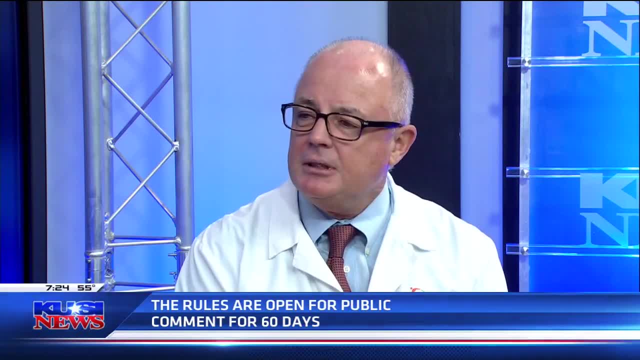 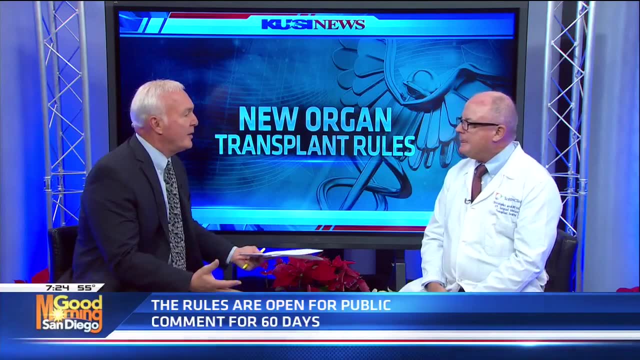 and you don't transplant an individual and they die. well, that doesn't help either. So those are three areas. Looking at your crystal ball, how's this all gonna change in 30 years' time? Are we gonna be creating the organs in a test tube? 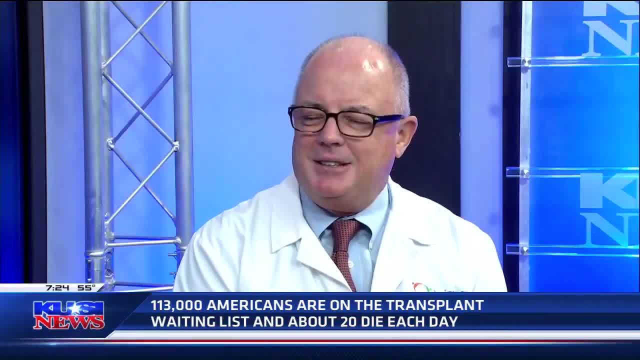 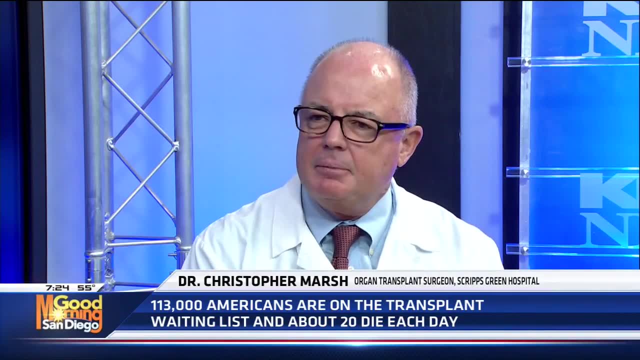 and there won't even be a need for living donors. Well, that's a good question. There's certainly work with stem cells to try and create organs, 3D printing things like that. Probably in the near future would be using genetically modified pigs organs. 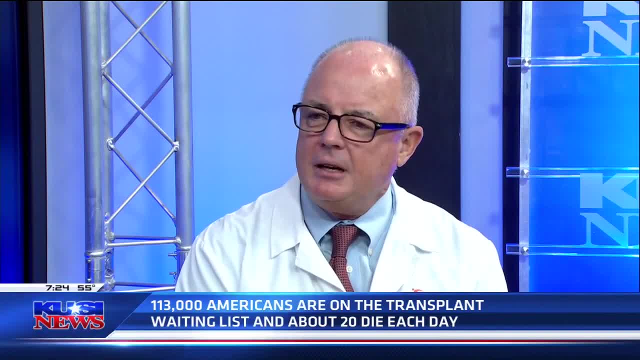 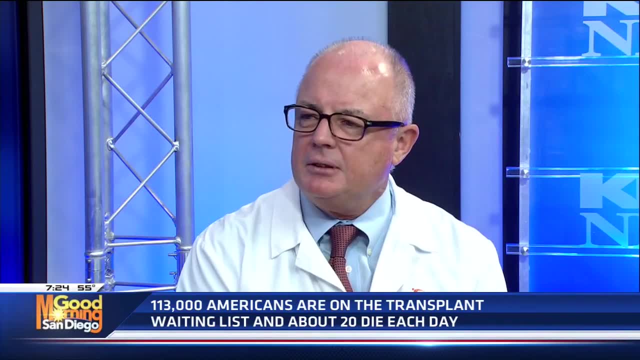 For certain valves and whatnot- heart valves, Like what we're doing for valves. but now they've modified pigs and knocked them out. Knocked out certain genes make them acceptable for human transplantation. All right, so Joe Blow at home. 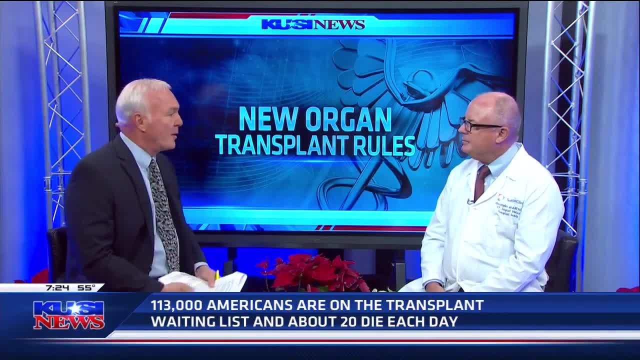 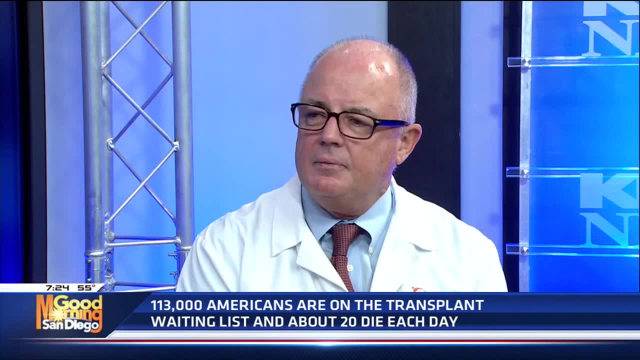 who is interested in this, either with a family member or close friend that is in need of an organ. How can we do we have any influence over the political process as far as these rules becoming into effect? Well, I think they're good. 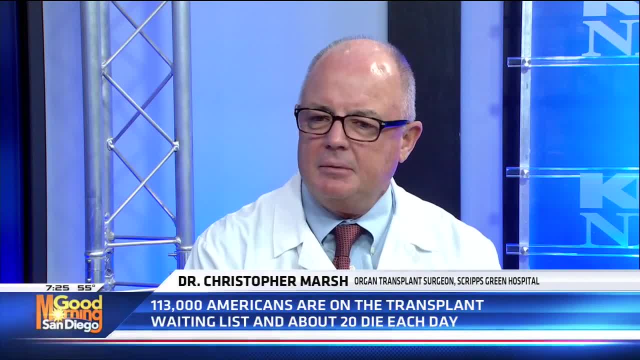 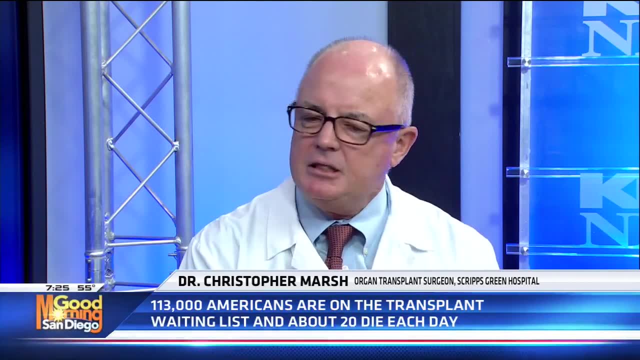 We'll see how this plays out, but I think they're good rules. I think. more importantly, I think people that wanna be an organ donor should step forward and at least be evaluated. Obviously there's reasons. they might not based upon social factors or just wage factors. 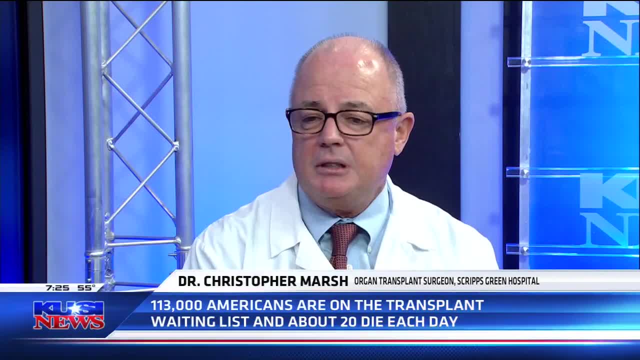 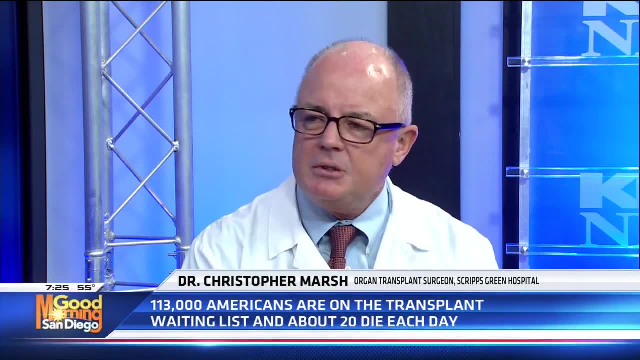 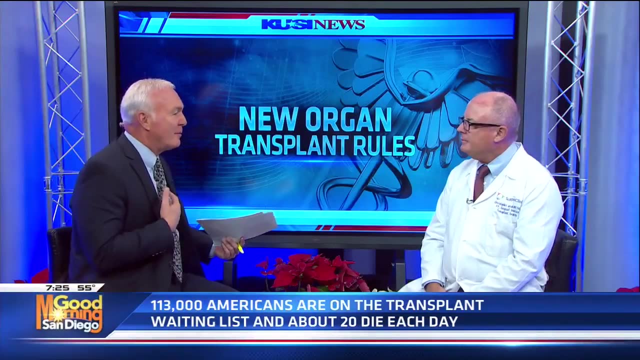 but I think, calling for Scripps, you could call and look into more information through scrippsorg or call 1-800-Scripps and get more information. but anyone can be a donor. I just the transplant technology just in my lifetime- has just made significant steps. 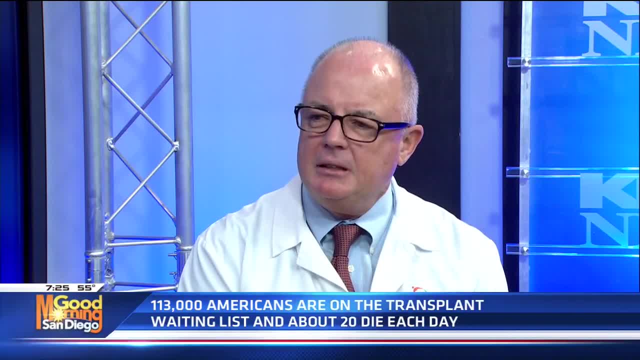 We do. we continue to. I mean, I think we're doing a very good job, but we need to continue to push. And I think at Scripps we're doing research in organ pumping and we're gonna be looking at stem cell.